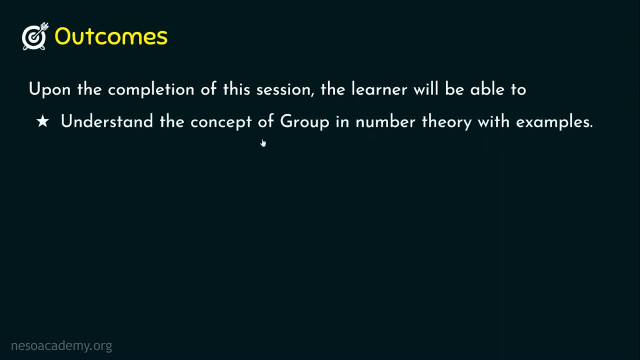 will be able to, outcome number 1, we will understand the concept of group in number theory with examples. Outcome number 2, we will understand the concept of abelian group 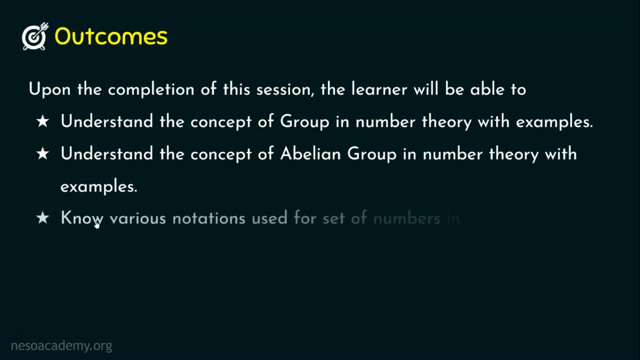 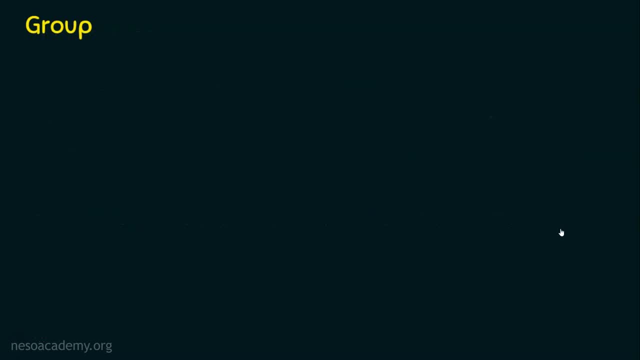 in number theory with examples. And outcome number 3, we will know various notations used for set of numbers in number theory. Let's dive into the topic of the day, the group. 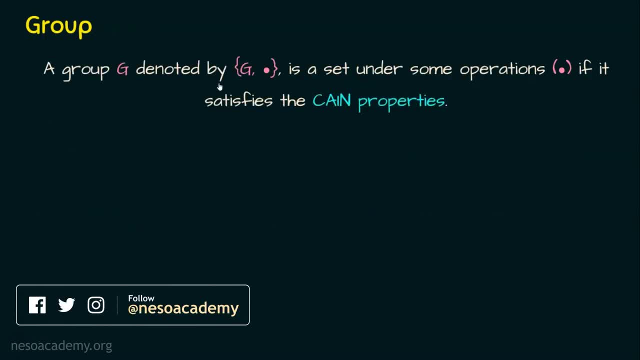 Firstly, let's see the definition. A group G denoted by G comma dot. It is a set under some operations dot. If it satisfies the C A I N properties. Before I explain the C A I N properties, let me first tell you, the group G denotes the set of numbers in number 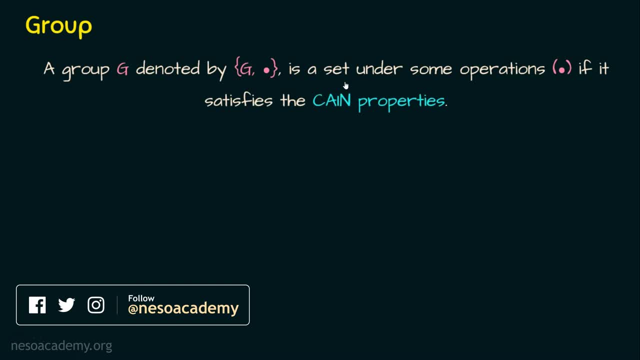 theory is a set, where it is going to contain a set of items. But this group is not referred as simply set. It is referred as group. Why it is referred as group? Because this set of elements under this operation dot, when it can satisfy these properties, then this set is called as a group. Now what are all the set of four properties, that is the C A I N properties to be satisfied for the set to be a group under the operation dot. The 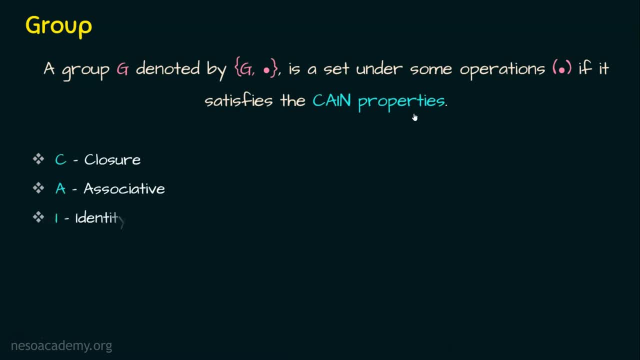 properties are C for closure, A for associative, I for identity and N for inverse. If these 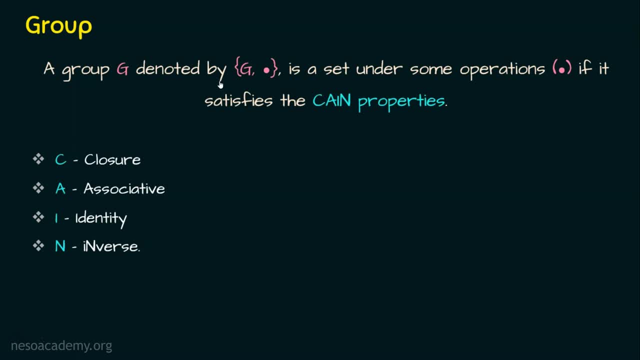 four properties are satisfied, then G comma dot is said to be a group. Please note here this dot is a binary operation. It's going to take two inputs and going to generate the 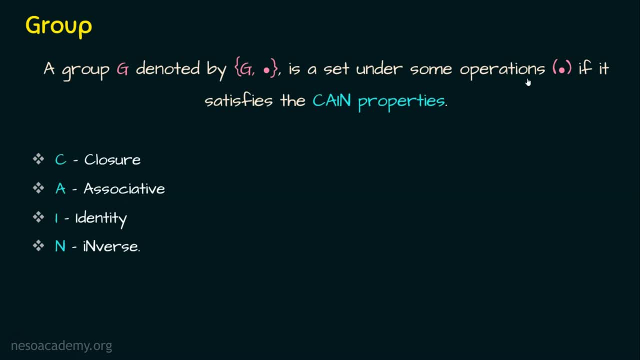 output. No worries, when we see an example, it will be easy for you. We are done with 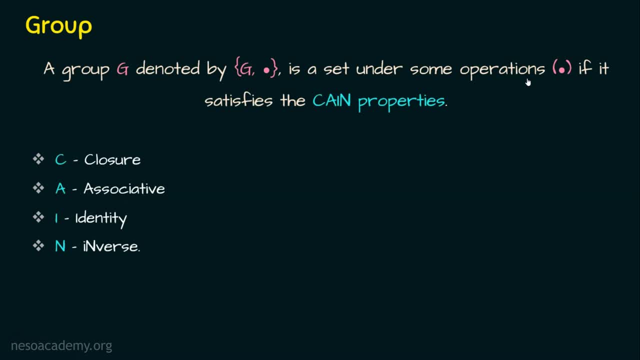 the definition of group. Let's now see the definition of a billion group. 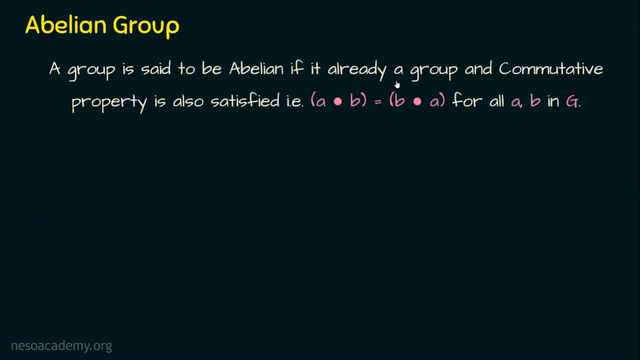 A group is said to be a billion if it is already a group and commutative property is also satisfied. A group is said to be a billion. Firstly, it should be a group. It means an abelian group should be satisfying these four properties closure, associative, identity and inverse. In addition to these properties, if the additional property that is the commutative property is also satisfied, then this group is said to be an abelian group. 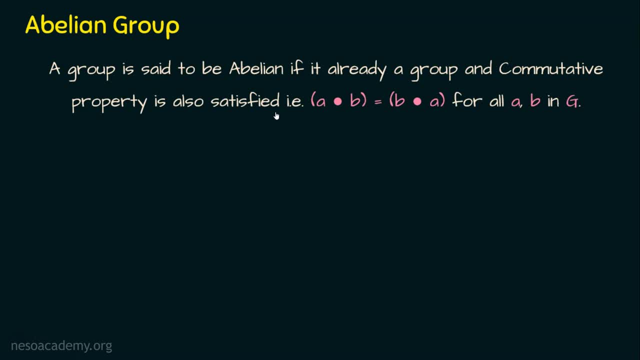 group should be satisfying these four properties: closure, associative identity and inverse. In addition to these properties. if the additional property, that is, the commutative property, is also satisfied, then this group is said to be an abelian group. What is this commutative property? Say a dot b is equal to b dot a for all, a comma b in. 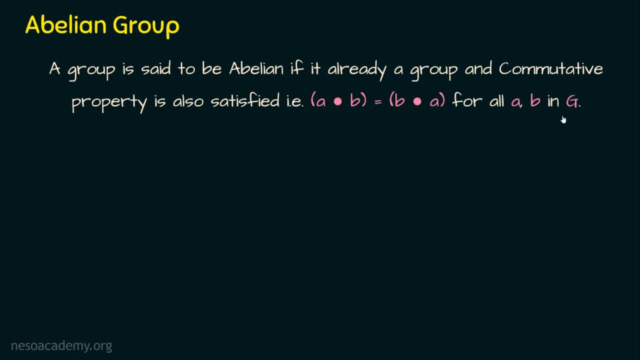 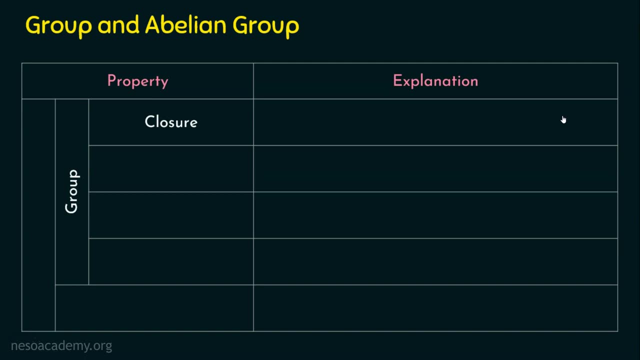 G. When we see an example, then it will be clear for you. So before stepping into the example, let's see the properties. If it is a group, then it should be satisfying closure property, associative property, identity element should exist and inverse element should also. 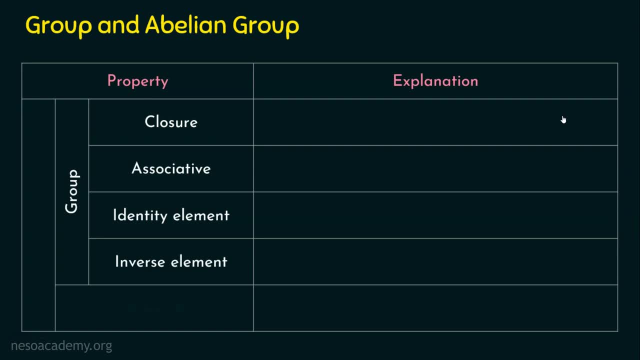 exist in the group In addition to these properties. if the additional property, that is, the commutative property, is also satisfied, then it forms an abelian group. Now let's see the explanation of each property. Let's first focus on the closure property. Let's take two elements, a comma b, that 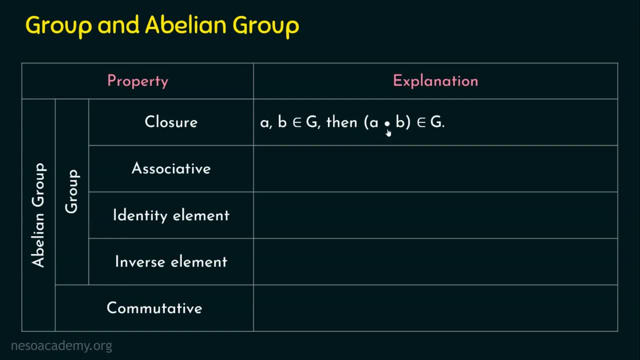 is belonging to the group g. If the a dot b operation we carry out and the result of this a dot b operation is also in the group, then closure property is satisfied. Then what is associative? a dot b, dot c is equal to a dot b, dot c for all the values of a comma b, comma c. that 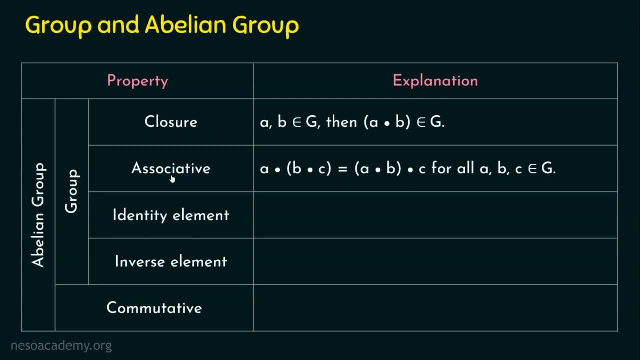 belongs to g. When this is satisfied, then associative property is also satisfied. Then what is identity element? Let's take an element a, When that element a is performed with the operation dot with the other element e, and when this a dot e or e dot a gives a again, then identity element. 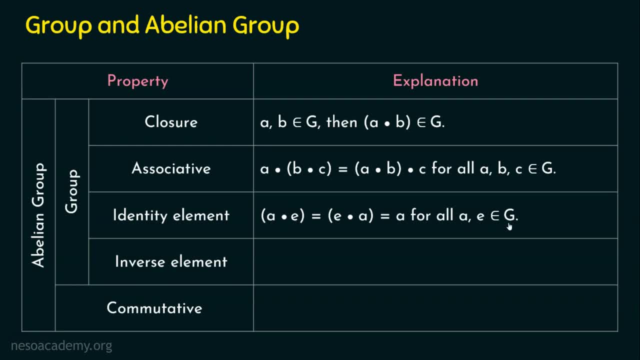 exists Where these a and e are also a part of the group. This is exactly identity element. and what's the next one? There exists an inverse element in the group. Say, if you take an element a and this a should have its inverse in the group, so that this element a and its inverse under this dot operation. 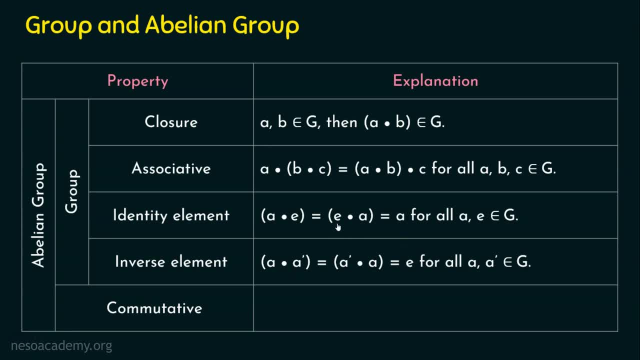 will give the identity element which we have seen in the previous property, which is the identity property. So when a dot, a dash, that is the inverse, when it gives the identity element for a comma, a dash which belongs to g, then there exists an inverse element. when these four 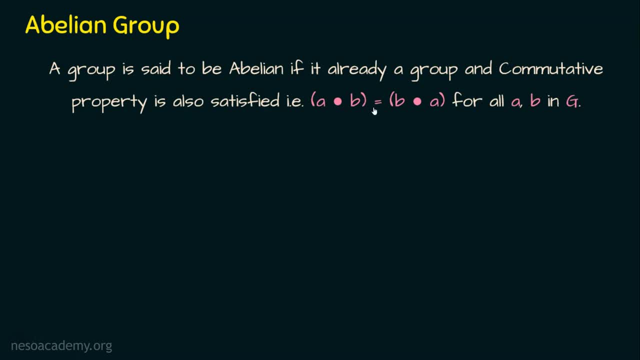 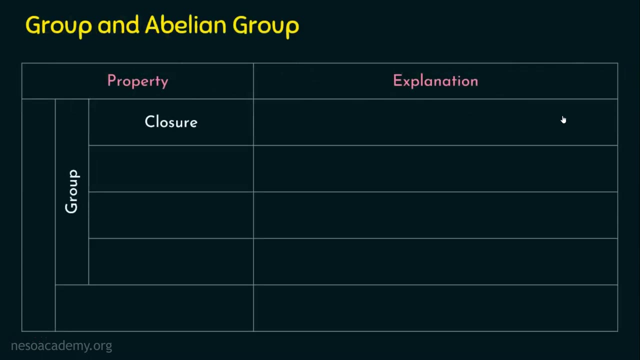 What is this commutative property? Say, A dot B is equal to B dot A for all A comma B in G. When we see an example, then it will be clear for you. So, before stepping into the example, let's see the properties. If it is a group, then it should be satisfying closure property, associative property, identity element should exist and inverse element should also exist in the group. In addition to these properties, if the additional property that is the commutative property is also satisfied, then this group is said to be a group. If 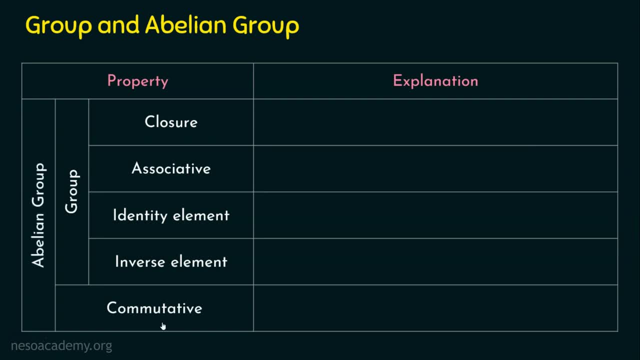 the commutative property is also satisfied, then it forms an abelian group. 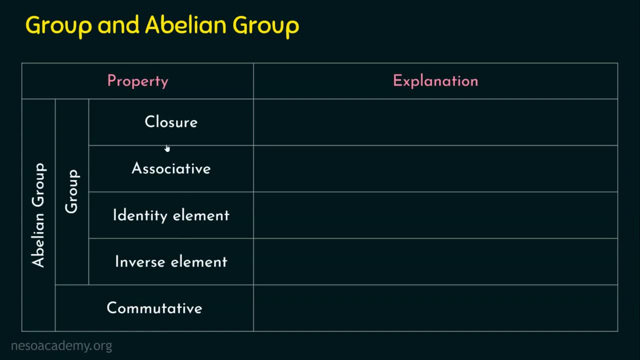 Now let's see the explanation of each property. Let's first focus on the closure property. Let's take two elements A comma B that is belonging to the group G. If the A dot B operation we carry out and the result of this A dot B operation is also in the group, then closure property is satisfied. Then what is associative? A dot B dot C is equal to A dot B dot C for the values of A comma B comma C that belongs to G. When this is satisfied, then associative property is also satisfied. Then what is identity element? Let's take an element A. When that element A is performed with the operation dot with the other element E and when this A dot E or E dot A gives A again, then identity element exist in the group where these A and 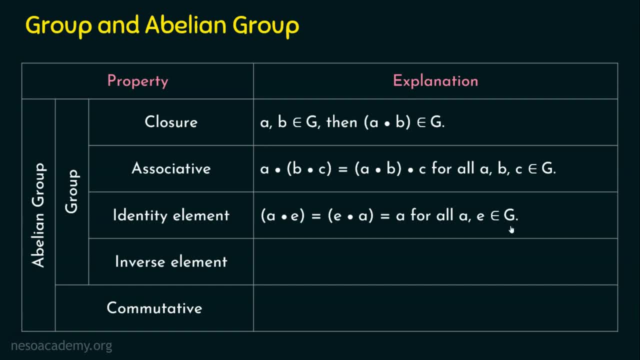 E are also a part of the group. This is exactly identity element. And what's the next one? There exist an inverse element in the group. Say if you take an element A and this A should have its inverse in the group so that this element A and its inverse under this dot operation will give the identity element which we have seen in the previous property which is the identity property. So when A dot A dash, that is the inverse, when it gives the identity element for A comma A dash which belongs to G, then there exist an inverse element. Then these four properties are given. 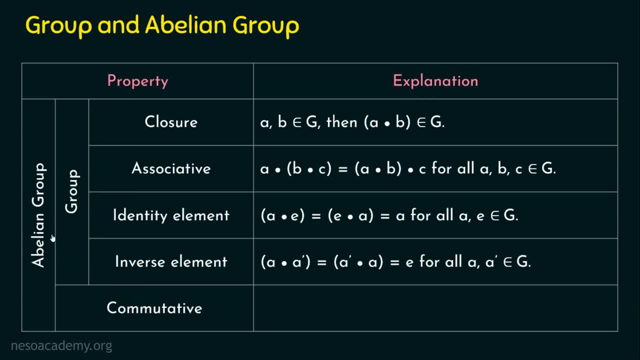 are satisfied, then it is a group. A group is said to be abelian if it is 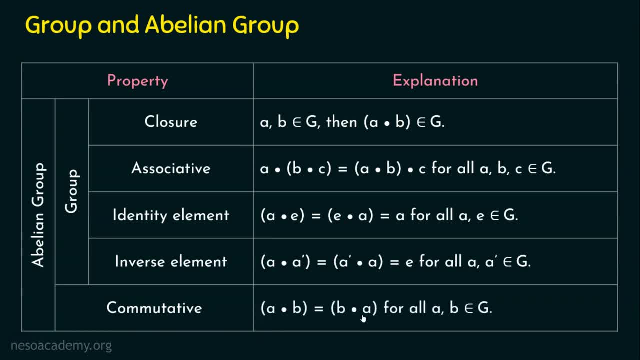 commutative. a dot b is equal to b dot a for all a comma b belongs to g. So we 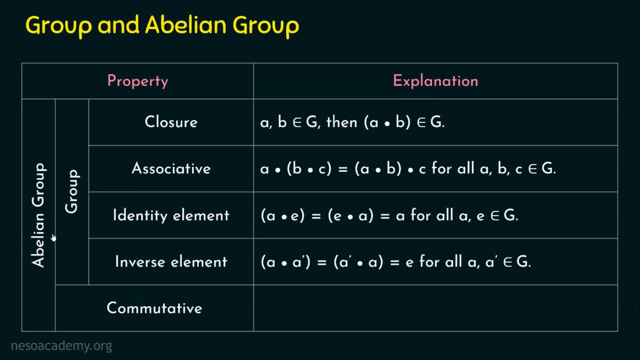 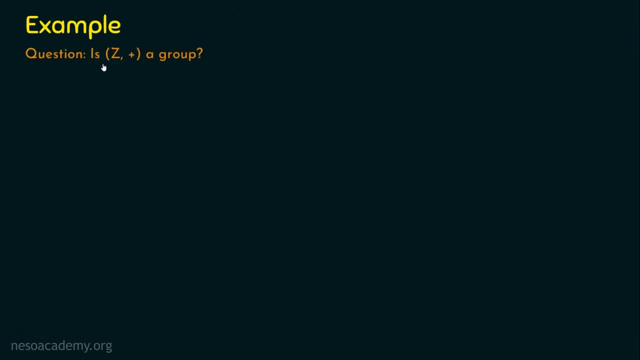 properties are satisfied, then it is a group. A group is said to be abelian. if it is commutative, a dot b is equal to b dot a for all. a comma b belongs to g. So we have seen the theoretical aspects of a group and abelian group. Let's see with an example. The question is: is z comma plus? 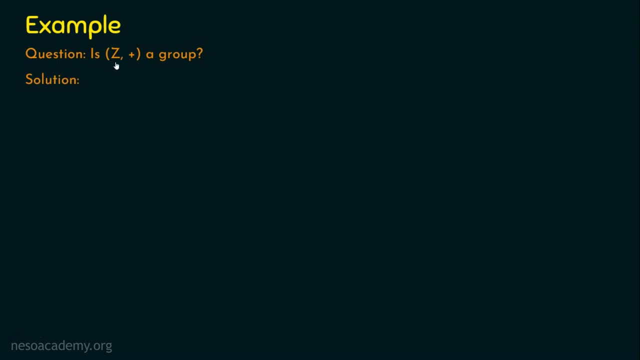 a group. Let's solve it now. What is this z? We know z means it's a set of integers. so this is the set of integers and this is actually a set. when we will call this set to be a group, when the four properties are satisfied, right? Let's see one by one now, Before. 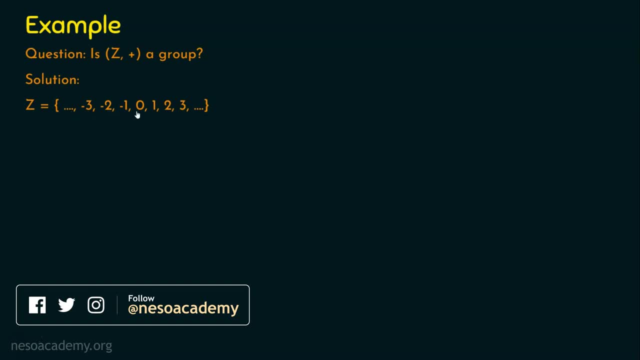 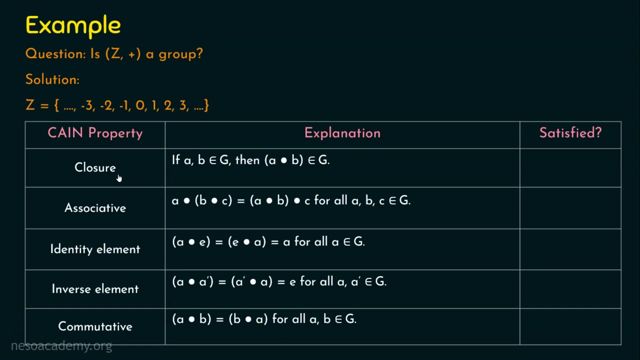 stepping into that. the set of integers are all negative numbers, zero and positive numbers are forming a set of integers which is represented as z. Now let's solve this. now We need the c, a, i, n property to be satisfied, right? Let me paste the properties now which we have seen in the previous. 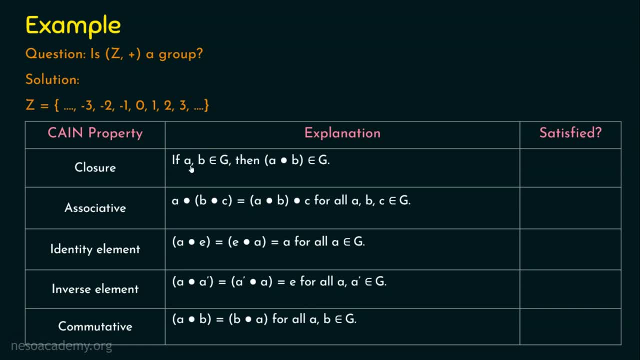 slide. Now let's deal with closure property. Let's take two elements a comma b from the group. See, we want to take the set of integers and we want to confirm whether it is a group or not. So what I am going to do is I am going to take two elements, a and b from this set which is belonging. 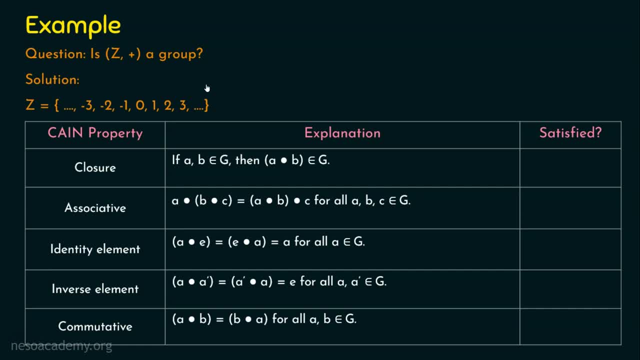 to this group, Then I am going to perform a dot b operation. Here the operation that is mentioned is plus. It is the addition operation. So we are going to check whether the set of integers and addition operation is forming a group or not. 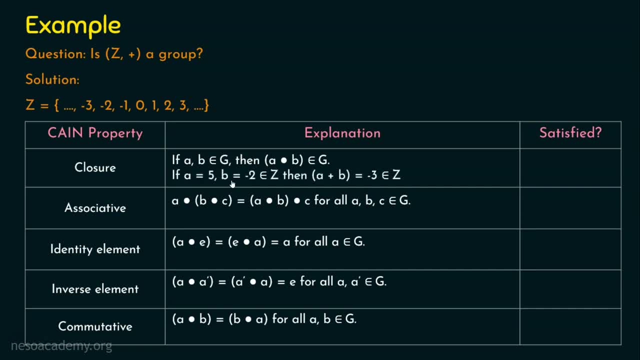 Let's take any two elements. Let me take here: a is equal to 5 and b is equal to minus 2, which belongs to z. right Now let's carry out the operation. What is the operation? a plus b? because the operation dot- here it is mentioned as plus 5 plus minus 2- will give minus 3 where minus 3 is. 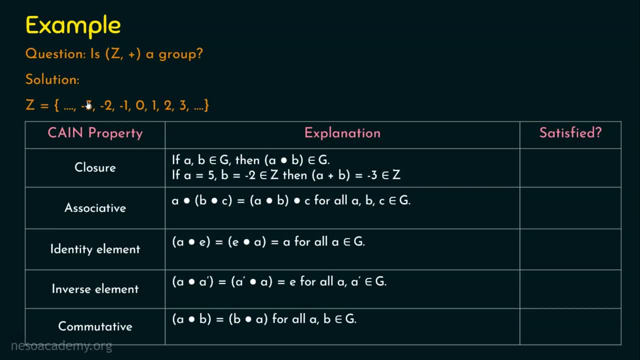 also belonging to z, because this minus 3 is also existing in the group. So the first property is getting satisfied, which is called as the closure property. Let's now move on to the second property, the association of the two elements. Let's take any two elements Let me take here: a is equal to 5 and b is. 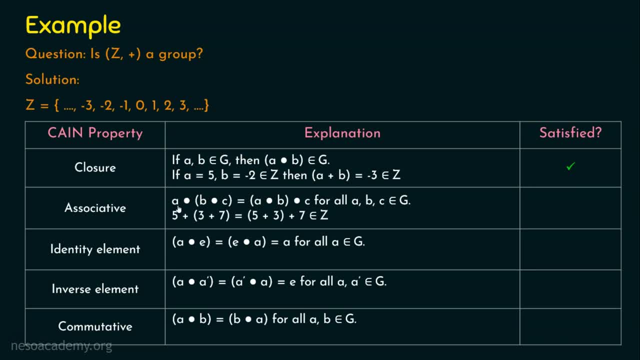 equal to 3 and c is equal to 7.. 5 plus 3 plus 7 is equal to 5 plus 3 plus 7.. Here we will have 15.. Here also we will have 15, where 15 is also belonging to this group, right. So obviously the 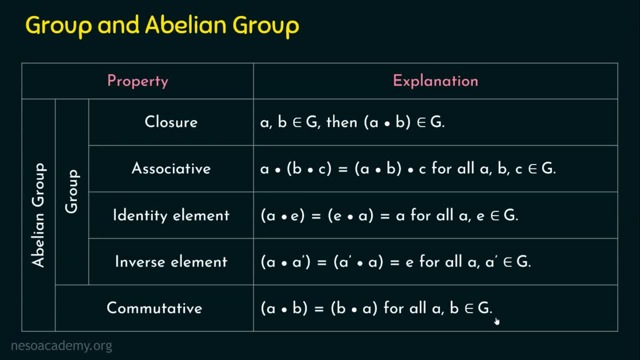 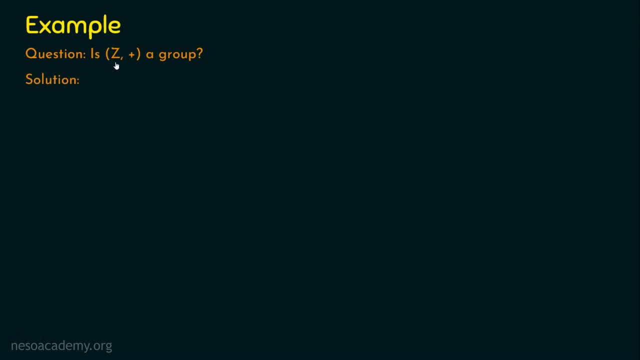 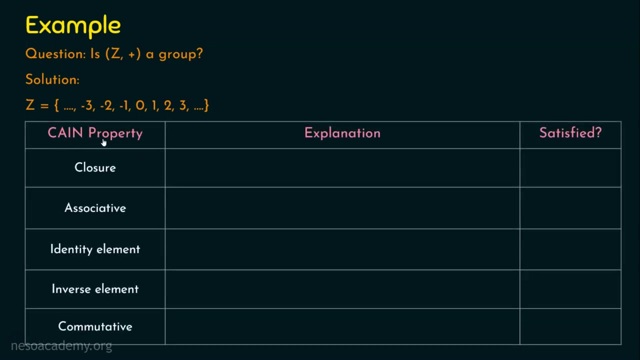 have seen the theoretical aspects of a group and abelian group. Let's see with an example. The question is, is z comma plus a group? Let's solve it now. What is this z? We know z means it's a set of integers. So this is the set of integers and this is actually a set. When we will call this set to be a group? When the four properties are satisfied, right? Let's see one by one now. Before stepping into that, the set of integers are all negative numbers, zero and positive numbers are forming a set of integers which is represented as z. Now let's solve this now. We need the c a i n property to be satisfied, right? Let me paste the properties now which we have seen in the previous slide. Now let's deal with closure property. 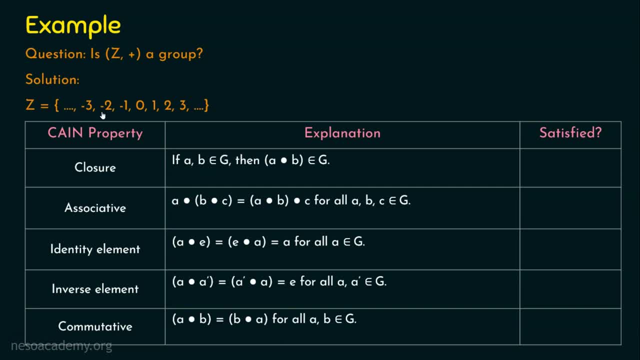 Let's take two elements a comma b from the group. See we want to take the set of integers and we want to confirm whether it is a group or not. So what I'm going to do is, I'm going to take two elements a and b from the set which is belonging to this group. Then I'm going to perform a dot b operation. Here the operation that is mentioned is plus. It is the addition operation. So we are going to check whether the set of integers and the addition operation is forming a group or not. Let's take any two elements. Let me take here a is equal to 5 and b is equal to minus 2 which belongs to z, right? Now, let's carry out the operation. What is the operation? a plus b because the operation dot here it is mentioned as plus. 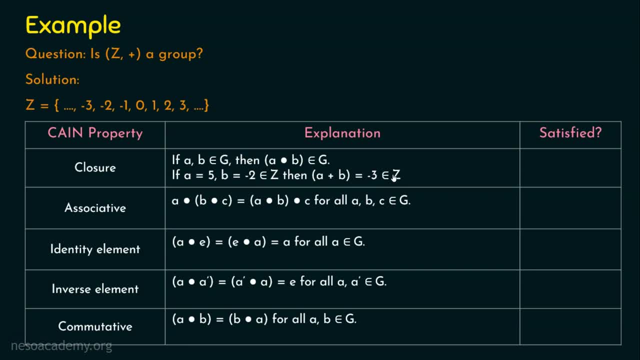 5 plus minus 2 will give minus 3 where minus 3 is also belonging to z because this minus 3 is 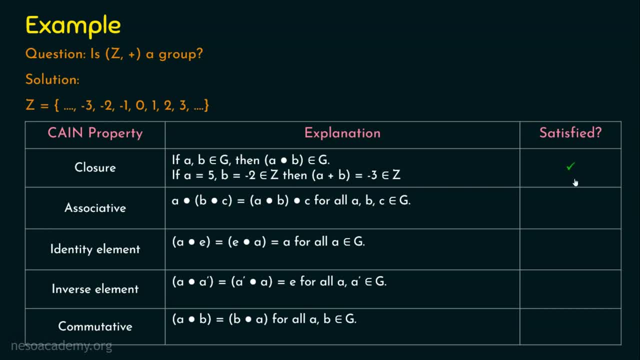 also existing in the group. So, the first property is getting satisfied which is called as the closure property. Let's now move on to the second property, the associative property. Let's take any numbers 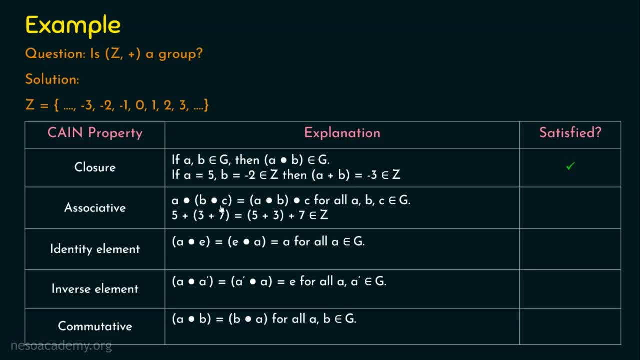 from the group. Let me take a is equal to 5, b is equal to 3 and c is equal to 7. 5 plus 3 plus 7 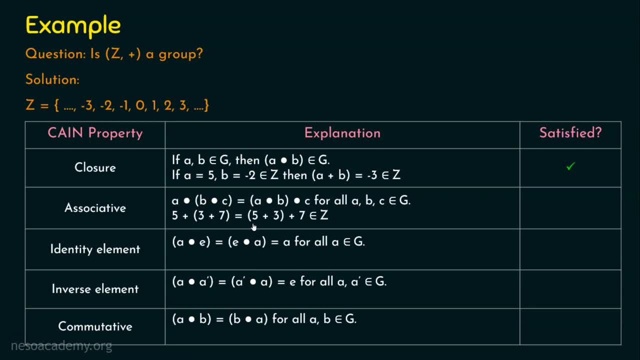 is equal to 5 plus 3 plus 7. Here, we will have 15. Here also, we will have 15 where 15 is also belonging to this group, right? So, obviously, the second property associative property is also 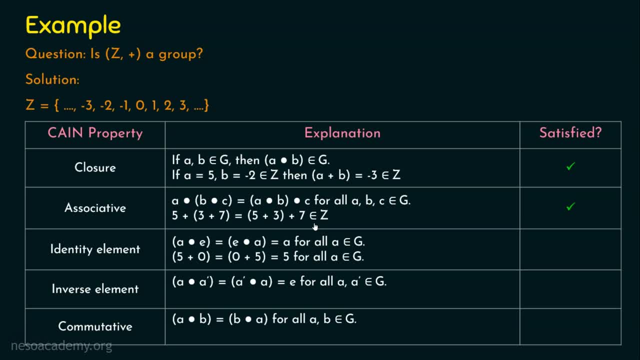 getting satisfied. Let's now move on to the third property. There exists an identity element. Say, when you take the number a, you have an identity element in this group 0 so that any number, under this operation, it will give the same number, right? So, 5 plus 0 is 5, 10 plus 0 is 10, 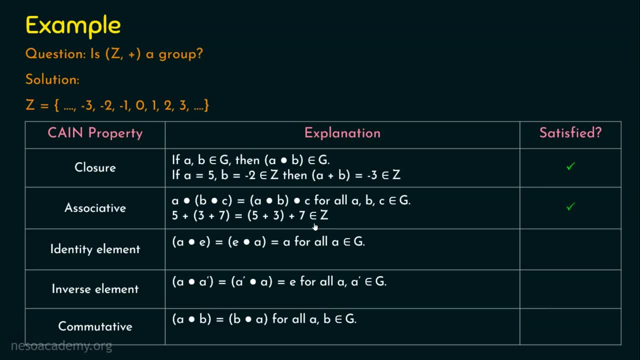 second property, associative property, is also getting satisfied. Let's now move on to the third property. There exists an identity element. Say, when you take the number a, you have an identity element in this group. So let's take the number a and b. Let's take the number a and b. Let's take the 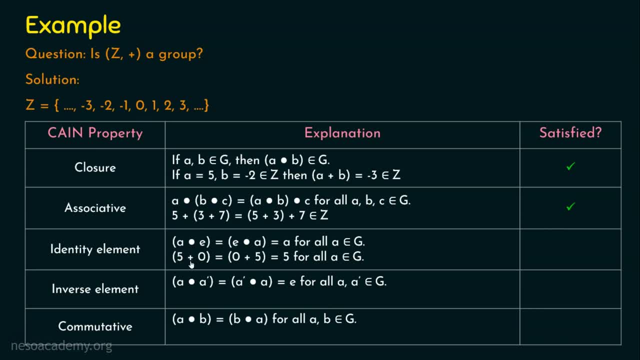 group 0 so that any number under this operation it will give the same number, right. So 5 plus 0 is 5, 10 plus 0 is 10,, 100 plus 0 is 100.. So you are getting the same number if you perform the. 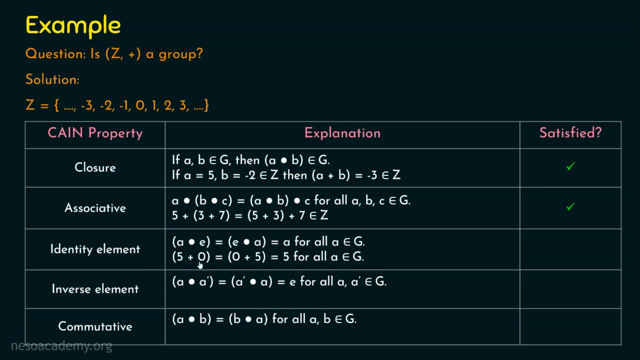 operation plus right. So there exists an element 0 which is also belonging to this group. So there exists an identity element in the group which is 0.. So the third property is also getting satisfied. Let's now move on to the fourth property, the inverse element. 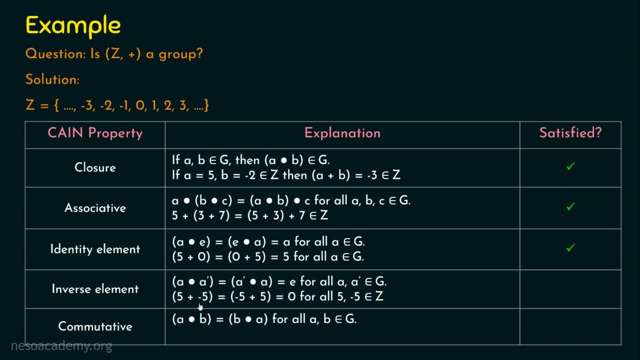 Does there exist an inverse element? Yes, if you take a number, 5, there exists minus 5.. So that 5 plus minus 5 will give 0, which is the identity element. right? You take any number, say 20 belongs to z. also minus 20 belongs to z, So that 20 plus minus 20 is 0, where 0 is the identity element. So from. 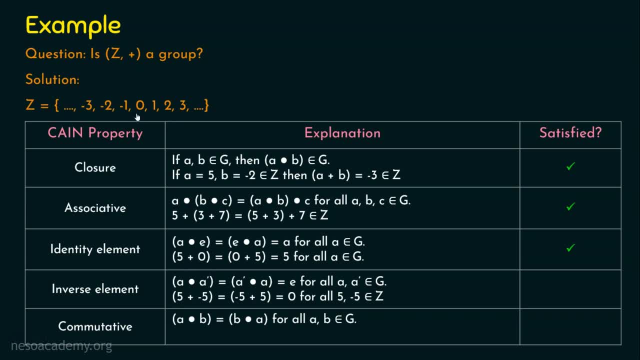 this we confirm that there exists an inverse element in z. So the fourth property is also getting satisfied. So it's clear that there is an inverse element in this group. So let's now move on to the fifth property. We have already figured that z comma plus is a group because it satisfies the 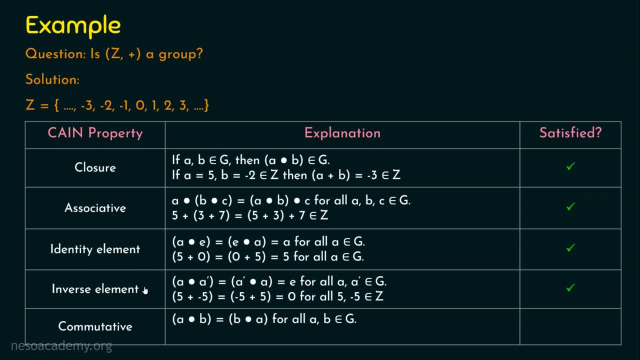 properties, closure, associative identity and inverse, which we simply refer it as cain properties or cain property. Already we have answered this question. z comma plus is a group. Now let's check whether it is an abelian group. If z comma plus to be an abelian group, then the fifth property. 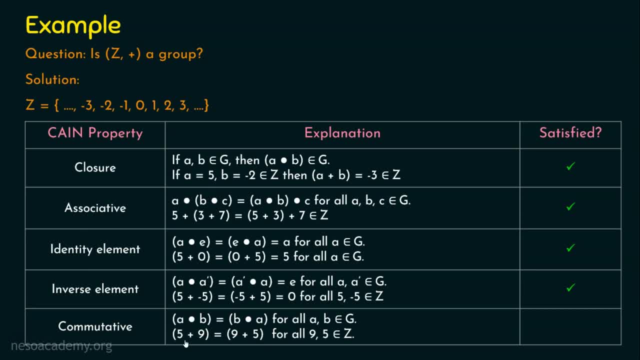 that is the commutative property, should be satisfied. Let's take any two numbers, 5 and 9, which is belonging to z. Now 5 plus 9 is equal to 9 plus 9.. So let's take any two numbers, 5 and 9. 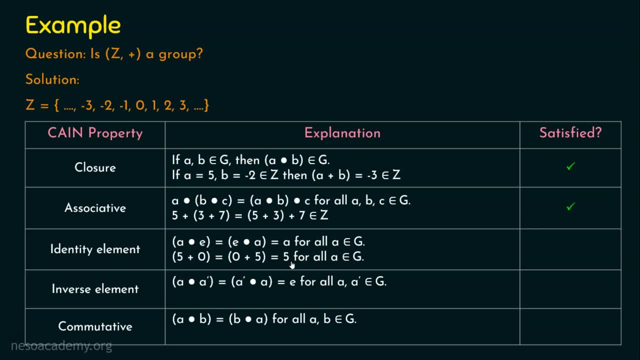 100 plus 0 is 100. So, you are getting the same number if you perform the operation plus, right? So, there exists an element 0 which is also belonging to this group. So, there exists an identity element in the group which is 0. So, the third property is also getting satisfied. 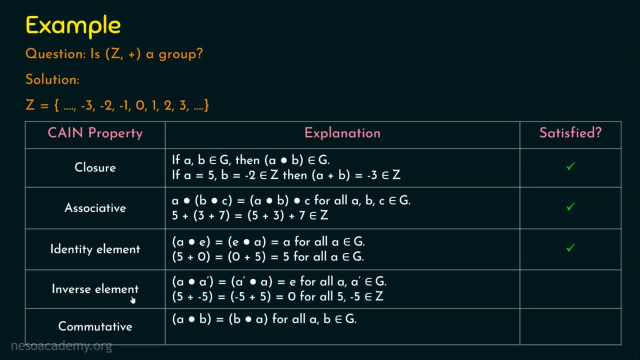 Let's now move on to the fourth property, the inverse element. Does there exist an inverse element? Yes. If you take a number 5, there exists minus 5. So, that 5 plus minus 5 will give 0 which is the identity element, right? You take any number. Say, 20 belongs to z. Also, minus 20 belongs to z. So, that 20 plus minus 20 is 0 where 0 is the identity element. So, from this, we confirm that there exists an inverse element in z. So, the fourth property is also getting satisfied. So, it's clear that z comma plus is a group. 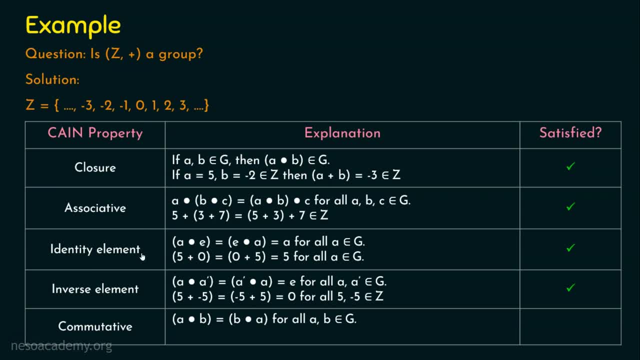 Because it satisfies the properties closure, associative, identity and inverse which we simply refer it as c-a-i-n properties or k-in property. Already, we have answered this question, 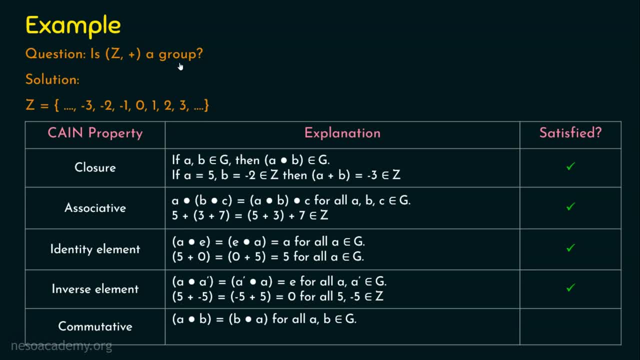 z comma plus is a group. Now, let's check whether it is an abelian group. If z comma plus to be an abelian group, then the fifth property that is the commutative property should be satisfied. 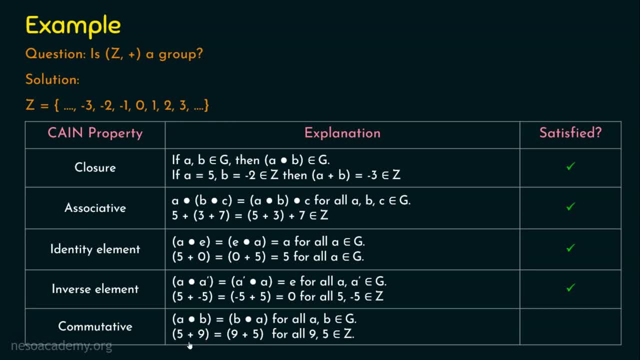 Let's take any two numbers 5 and 9 which is belonging to z. Now, 5 plus 9 is equal to 9 plus 5 obviously. And the result which is 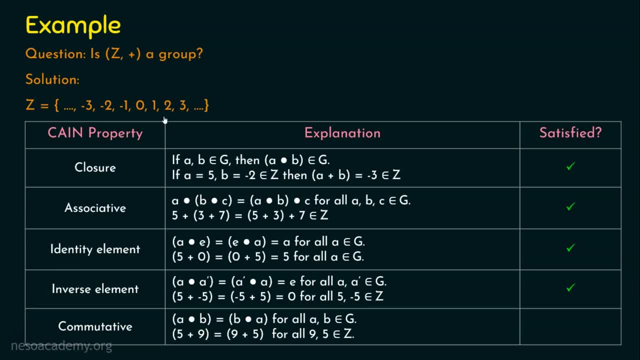 14 which is also belonging to this set, right? So, obviously, the fifth property, commutative property is also getting satisfied. We can say z comma plus is an abelian group. The answer for this question is z comma plus is a group and also it is an abelian group. In this example, 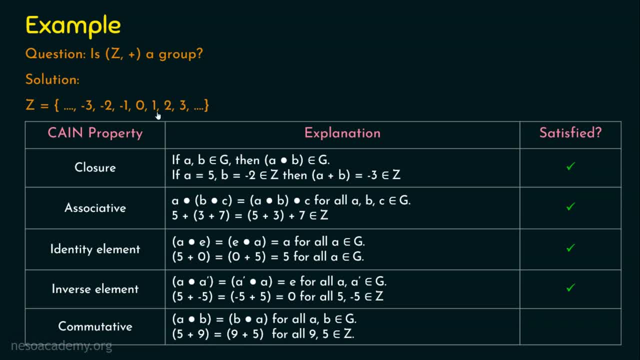 plus 5, obviously, and the result, which is 14, which is also belonging to this set right. So obviously the fifth property, commutative property, is also getting satisfied. We can say z comma plus is an abelian group. The answer for this question is z comma plus is a group and also it is an abelian. 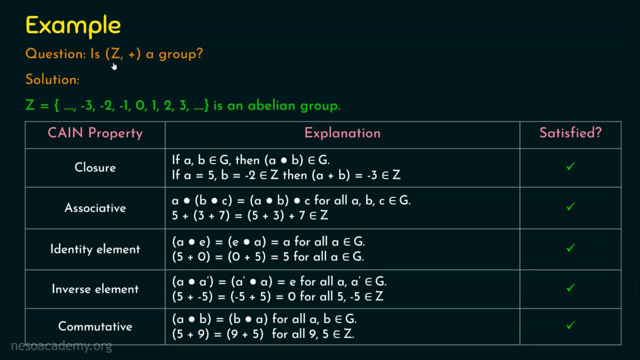 we have seen z as one of the notations. Let's see what are all the various notations we have in number theory. See, we have many notations here. n means it's the set of natural numbers. 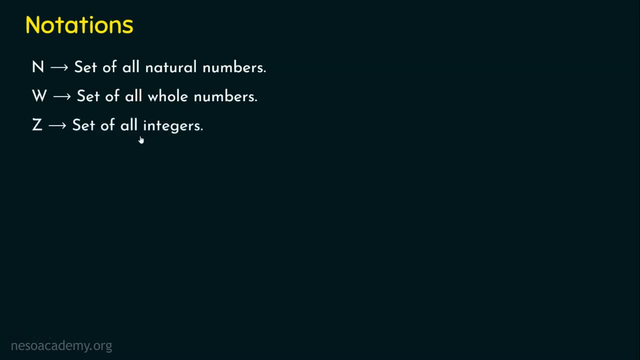 W means it's the set of whole numbers. Z means set of integers. C means set of complex numbers. Q means set of rational numbers. 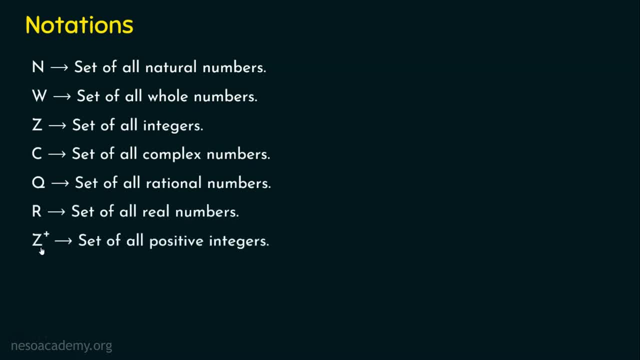 R means set of real numbers. Z plus means it's the set of positive integers only.